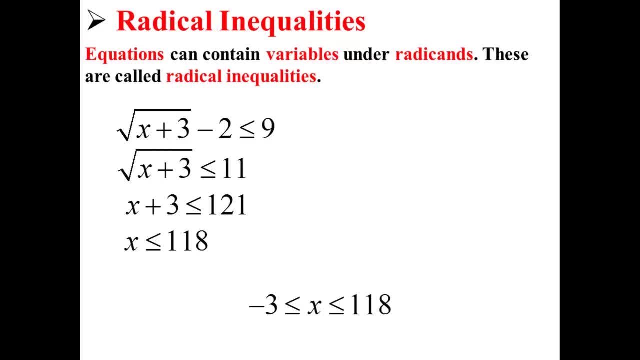 So our solution is: x must be greater than negative 3.. But we subtract 3 to get x is less than or equal to 118.. Sorry, greater than or equal to negative 3, but less than or equal to 118.. Let's try that out with a few values. 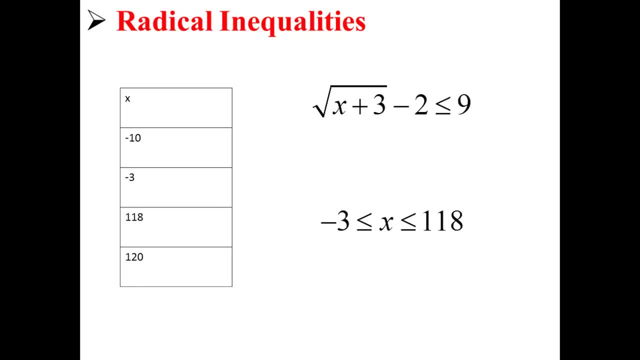 Here we're going to test the values negative 10,, negative 3,, 118, and 120 to make sure that we found the right answer. First we test the value negative 10.. This already isn't a solution, because that gives us the radical of negative 7,, which doesn't work. 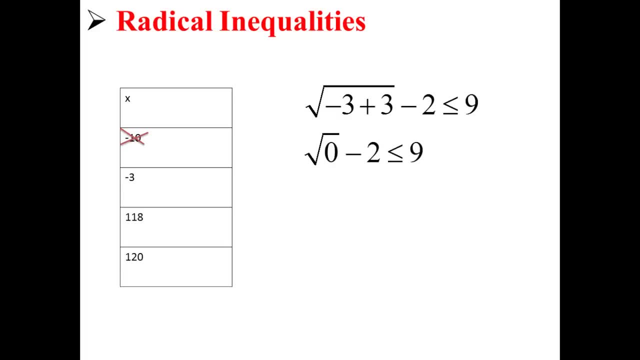 Next we test negative 3.. This gives us rad. 0 minus 2 is less than or equal to 9.. So negative 2 is less than or equal to 9.. This is a valid solution, so negative 3 works as an x. 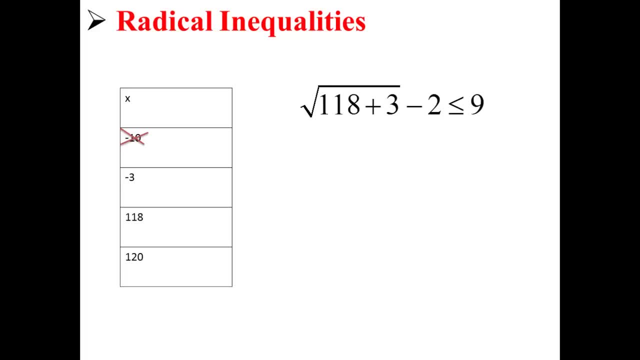 Next we try 118.. Radical 118 plus 3 minus 2 is less than or equal to 9.. That is to say that rad 121 minus 2 is less than or equal to 9.. This simplifies to: 11 minus 2 is less than or equal to 9, or simply 9 is less than or equal to 9.. 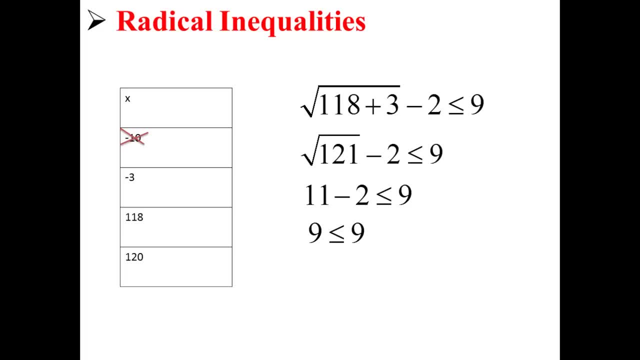 This is true, so 118 is a valid solution to our equation. Now let's try 120.. This gives us rad 123 minus 2 is less than or equal to 9, or 11.09 minus 2 is less than or equal to 9,, or simply 9.09 is less than or equal to 9.. 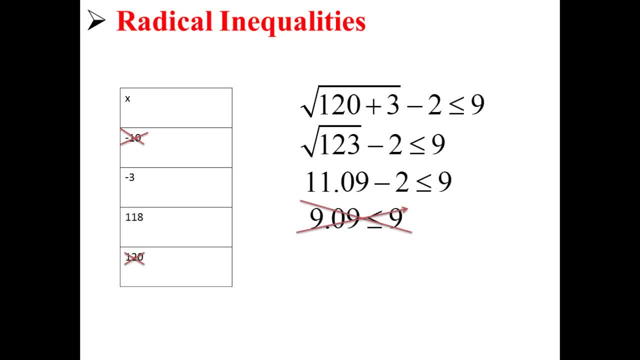 This answer also does not work. So values less than negative 3 don't work and values greater than 118 do work. So we know that our original solution- x is greater than or equal to negative 3, and x is less than or equal to 118,- is correct. 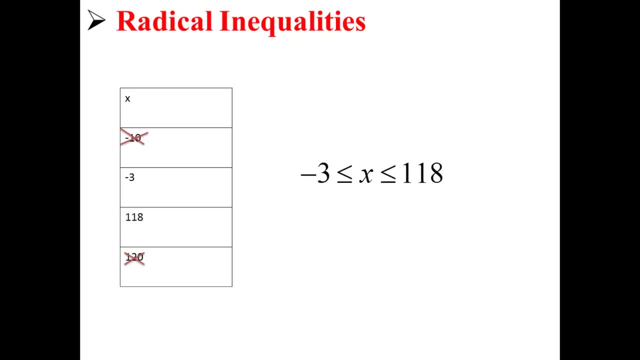 Any values within that range will be a valid solution to our radical inequality. Thank you for watching.